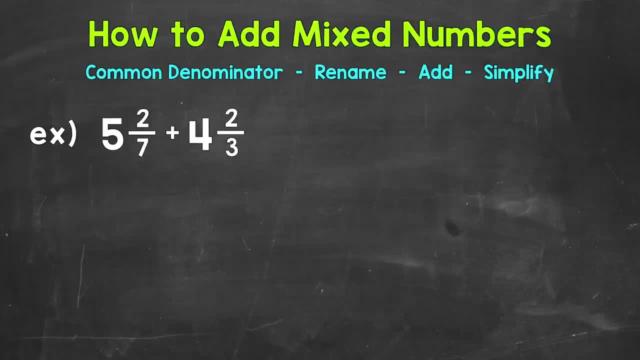 or examples, I dropped links to other videos on mixed numbers down in the description. Now, we're going to start with addition. Let's jump into our example where we have 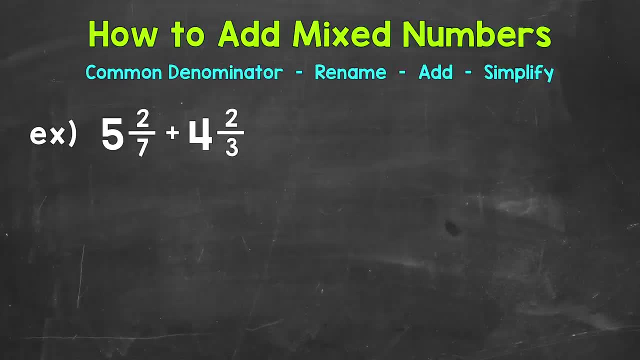 5 and 2 sevenths plus 4 and 2 thirds. Now, the first thing that I'm going to do, I'm going to rewrite this problem vertically, so up and down, lining up the fractions and whole numbers. So, we'll start with 5 and 2 sevenths, plus 4 and 2 thirds. So, once we do that, we need to find a common denominator. We're not able to add because we have a 7 and a 3 for our denominators. We need a common denominator in order to add the fractional part of these mixed numbers. So, in order to find a common denominator, we need to find a logarithm. 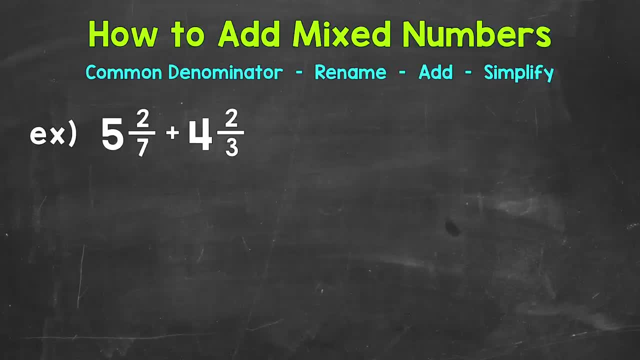 I'm going to rewrite this problem vertically, so up and down, lining up the fractions and whole numbers. So we'll start with 5 and 2 sevenths plus 4 and 2 thirds. So once we do that, we need to find a common denominator. We're not able to. 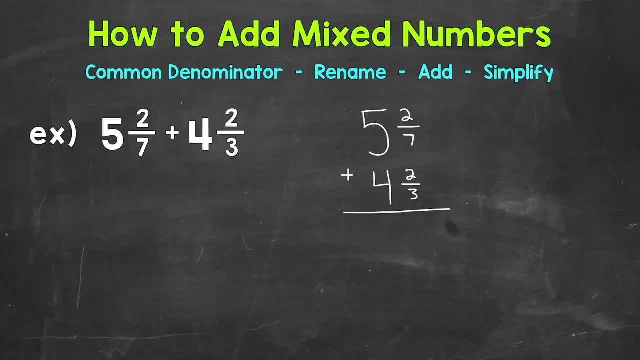 add, because we have a 7 and a 3 for our denominators, We need a common denominator in order to add the fractional part of these mixed numbers. So, in order to find a common denominator, we need to find a least common multiple, and that's going to be our least common denominator. Now you may be able to. 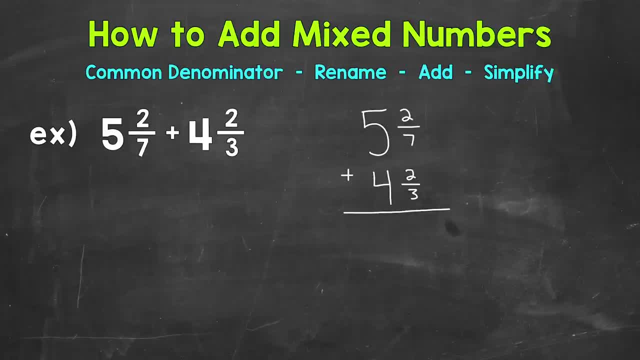 figure out what the least common multiple between 7 and 3 is without writing out the multiples. but as a review, I'm going to come to the side here and we'll write out our multiples and I'll show you how to find the least common multiple. And again, that's going to be our least. 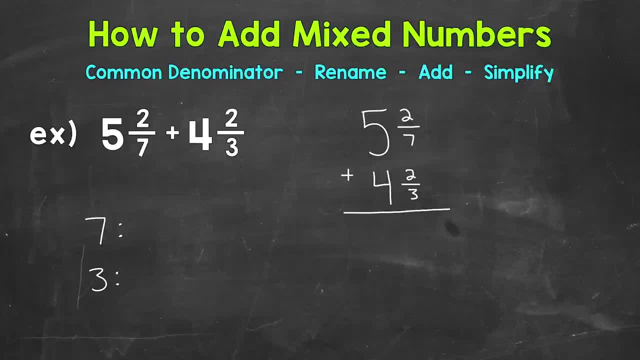 common denominator. So let's start with 7, and I'm going to write out the first 4 multiples of 7.. Now the multiples go on forever. so my suggestion: write 4 or 5. See if you have any in common. If not, you can always extend your lists. So 7,, 14,, 21,, 28.. 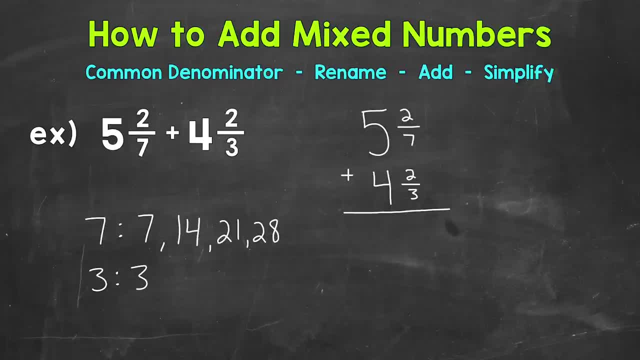 Now we'll write the first 4 multiples of 3.. So 3, 6,, 9,, 12., 12: we don't have any matches there. We don't have anything in common. So let's extend our lists. 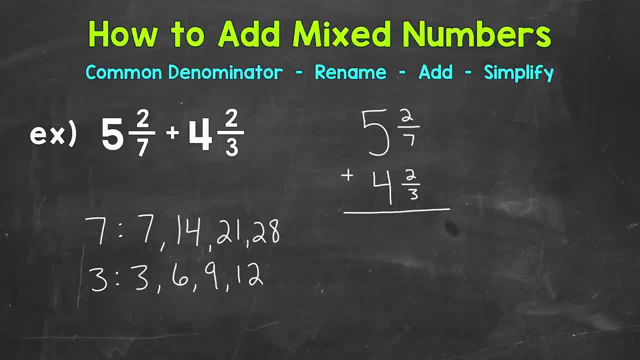 Now seven, we're already at 28. And for our multiples of three, we're only at 12.. So let's extend that list. So then we have 15,, 18,- still nothing in common- And then we have 21.. So 21. 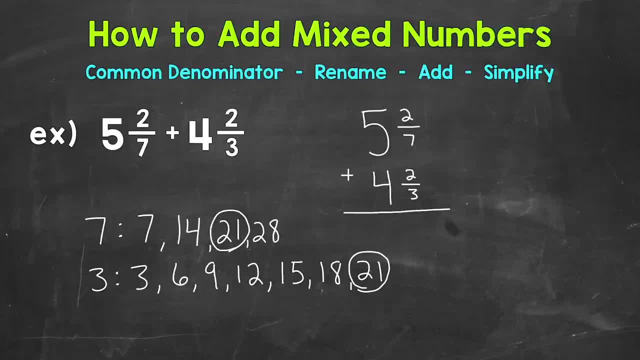 is going to be our least common multiple and therefore our least common denominator, So that's what we're going to use. So once we have that common denominator, we're going to rename the fractional part of our mixed numbers with that common denominator. That way we'll be able to add. 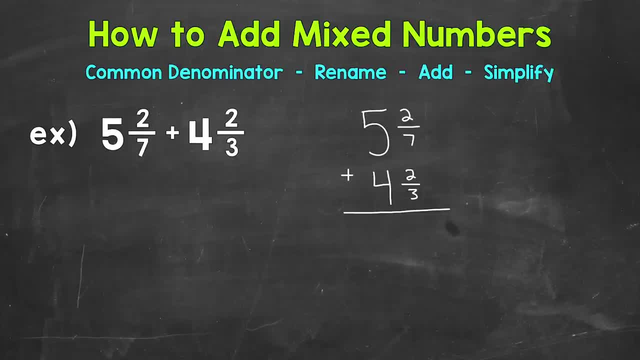 least common multiple. And that's going to be our least common denominator. Now you may be able to figure out what the least common multiple between seven and three is without writing out the multiples. But as a review, I'm going to come to the side here and we'll write out our multiples and I'll show you how to find the least common multiple. And again, that's going to be our least common denominator. So let's start with seven. And I'm going to write out the first four multiples of seven. Now the multiples go on forever. So my suggestion, write four or five. See if you have any in common. If not, you can always extend your lists. So seven, 14, 21, 28. Now we'll write the four multiples of three. So three, six, nine, 12. And we don't have any matches there. We don't have anything in common. So let's extend our lists. Now seven, we're already at 28. And for our multiples of three, we're only at 12. So let's extend that list. So then we have 15, 18, still nothing in common. And then we have 21. So 21 is going to be our least common multiple and therefore our least common denominator. So that's what we're going to use. So once we have that common denominator, we're going to rename the fractional part of our mixed numbers with that common denominator. That way we'll be able to add. So let's go over to our 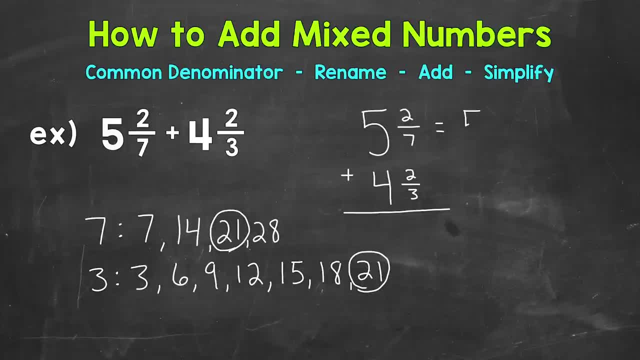 mixed numbers here and rename. We do not need to do anything with the whole numbers. So this is going to be 21. 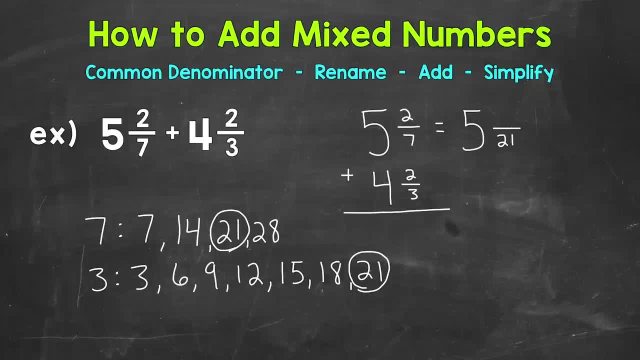 So let's use equivalent fractions to rename that to seventh with a denominator of 21. So we need to think, how do we get seven to equal 21? Well, seven times three is 21. Whatever we do to the bottom, we must do to the top. In order to keep this equivalent. Two times three is six. So six 21st's is equivalent to 2 7ths. We're not changing the number of sevens. We're not changing the number of sevens in our mixed numbers. Now if we 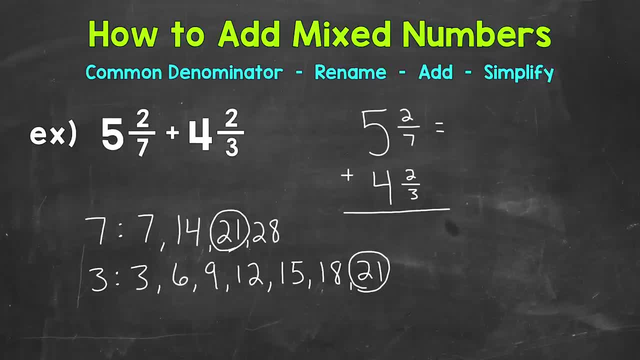 So let's go over to our mixed numbers here and rename- We do not need to do anything with the whole numbers- So this is going to be 21.. So let's use equivalent fractions to rename that two-sevenths with a denominator of 21.. So we 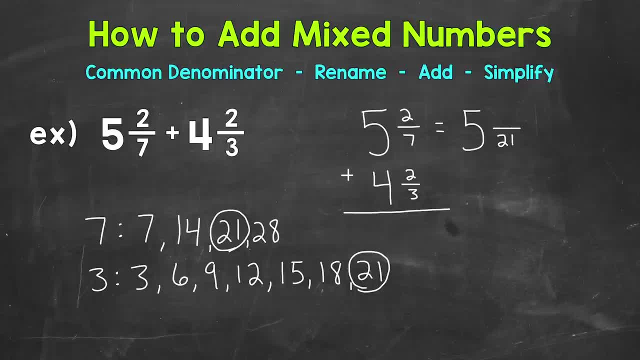 need to think: how do we get 7 to equal 21?? Well, 7 times 3 is 21.. Whatever we do to the bottom, we must do to the top in order to keep this equivalent. 2 times 3 is 6.. So 6, twenty-firsts. 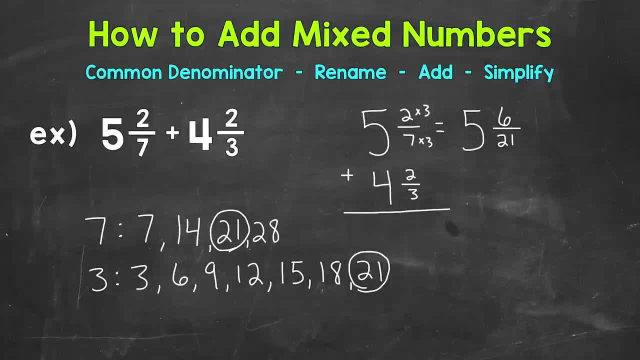 is equivalent to 2.. We're not changing the value of the problem at all. These are equivalent fractions. We're just renaming using that common denominator. Let's bring the addition sign over and then we need to do 4 and two-thirds Again. we do not need to do anything with the whole number and we have a. 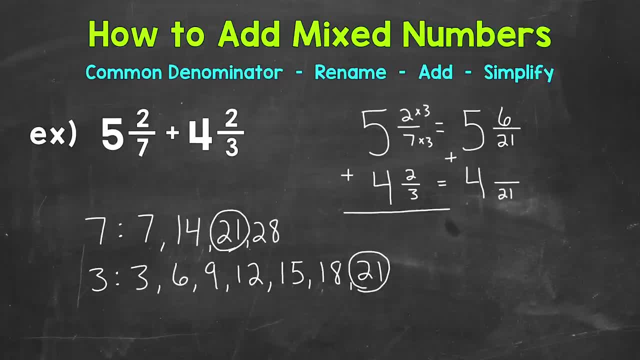 common denominator of 21.. So let's think: how do we get 3 to equal 21?? Well, 3 times 7 is 21.. Whatever we do to the bottom, we must do to the top in order to keep this equivalent. So 2 times 7 is 14.. So now we're ready to add To. 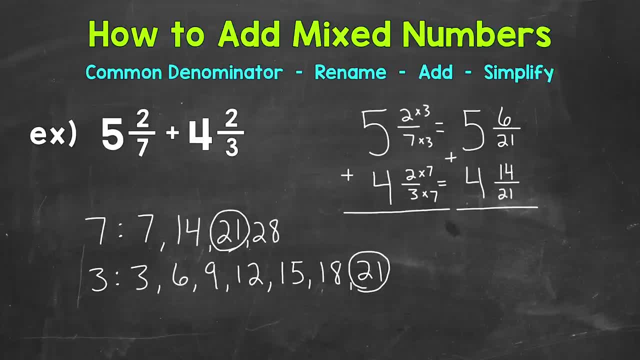 recap, we found our common denominator of 21,. then we renamed the fractions of our mixed numbers using that common denominator of 21.. Now that we have a common denominator between our fractions, we're able to add. So let's add our fractions and then whole numbers. 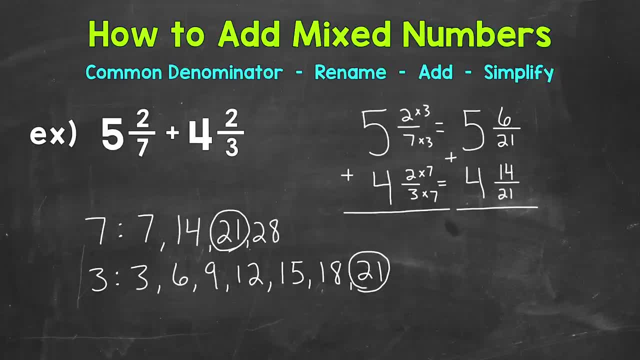 So for our fractions add the numerators: 6 plus 14 is 20.. And then we keep our denominator of 21.. So 6 twenty-firsts plus 14 twenty-firsts equals 20 twenty-firsts. So we added our fractions. 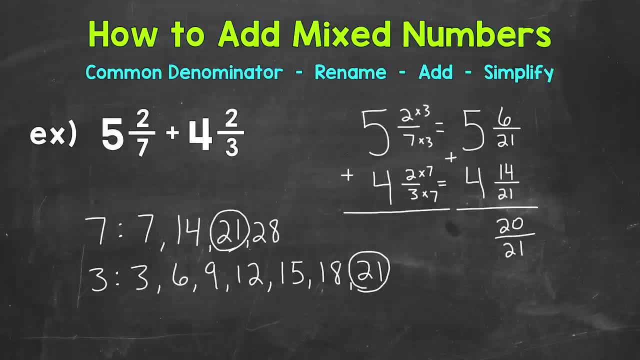 Now let's add the whole numbers. So 5 plus 4 is 9.. So our final answer is 9 and 20 twenty-firsts. Always check to see if you can simplify the fractional part of a mixed number. Well, 20 twenty-firsts is in simplest form. The only common factor between 20 and 21 is 1.. So we are. 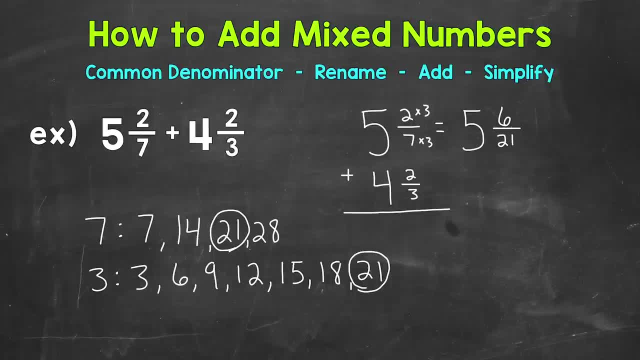 the value of the problem at all these are equivalent fractions we're just renaming using that common denominator let's bring the addition sign over and then we need to do four and two thirds again we do not need to do anything with the whole number and we have a common denominator of 21 so let's think how do we get 3 to equal 21 well 3 times 7 is 21 whatever we do to the bottom we must do to the top in order to keep this equivalent so 2 times 7 is 14 so now we're ready 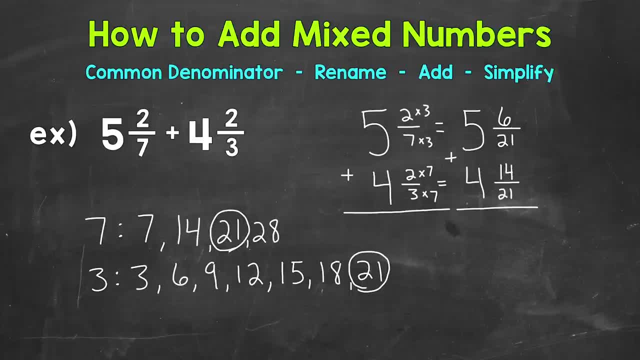 to add to recap we found our common denominator of 21 then we renamed the fractions of our mixed numbers using that common denominator of 21 now that we have a common denominator between our fractions we're able to add so let's add our fractions 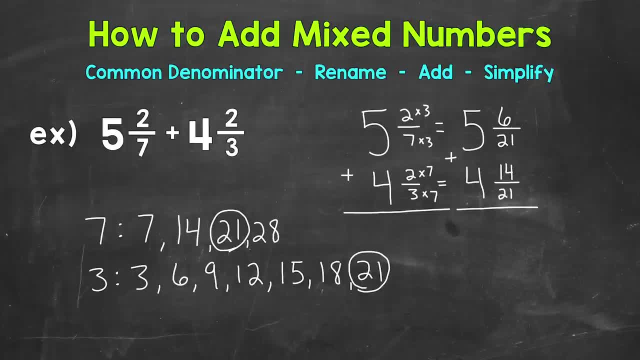 and then we're ready to add the common denominator of 21 and then we're ready to add the common denominator of 21 whole numbers so for our fractions add the numerators 6 plus 14 is 20 and then we keep our denominator of 21 so 6 21st plus 14 21st equals 20 21st so we added our fractions now let's add the whole numbers so 5 plus 4 is 9 so our final answer is 9 and 20 21st always check to see if you can simplify the fractional part of a mixed number well 20 21st is in simplest form the only common factor between 20 and 21 is 1 so we are done and our final answer 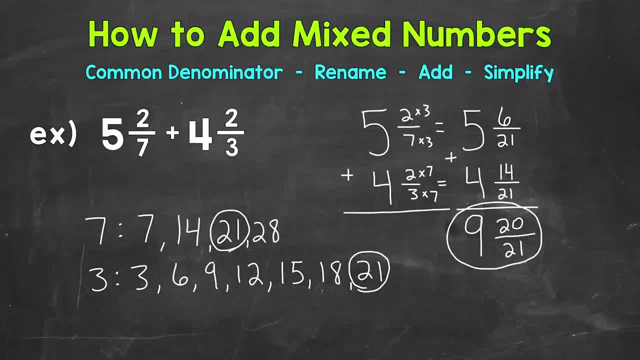 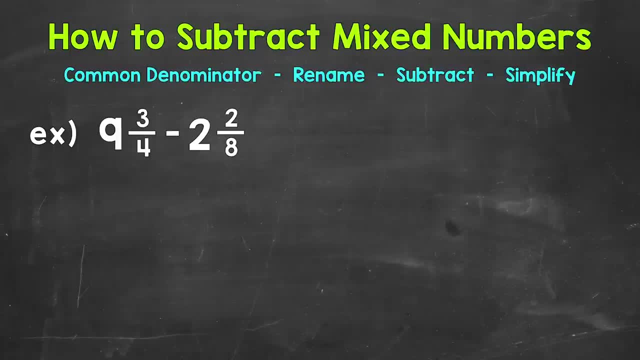 done And our final answer is 9 and 20- twenty-firsts. Next let's move on to subtraction. So for our subtraction example, we have 9 and three-fourths minus 2 and two-eighths. Now the first thing that I'm going to do is rewrite this problem. 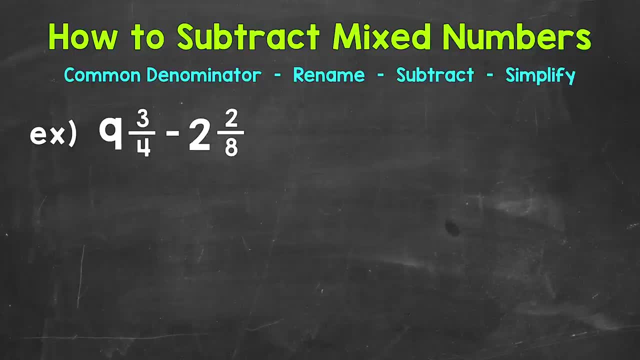 vertically, So up and down, And I'm going to line up my whole numbers and fractions. So let's come to the side here and we'll do 9 and three-fourths minus 2 and two-eighths. So what I'm going to do, I'm going to subtract the fractions first. 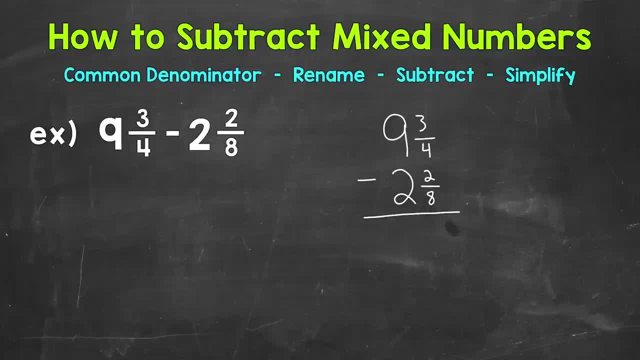 and then the whole numbers. Now, when we subtract fractions, we need a common denominator. So, as we have the problem written out now, we have a denominator of 4 and a denominator of 8. So we can't subtract quite yet. We need to find a common denominator and rename. We find a common. 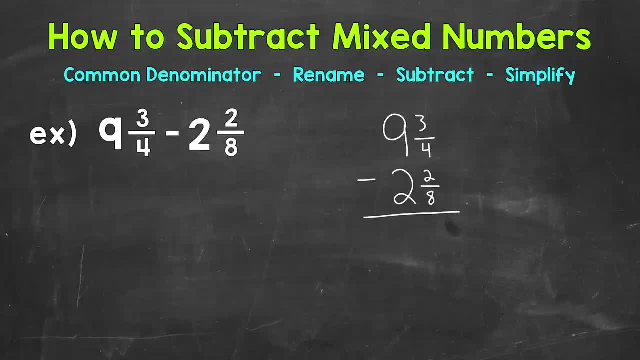 denominator by looking for common multiples And then the least common multiple we can use for our least common denominator. So let's write out our multiples of 4 and 8. Now you may be able to do this: figure out what the least common. 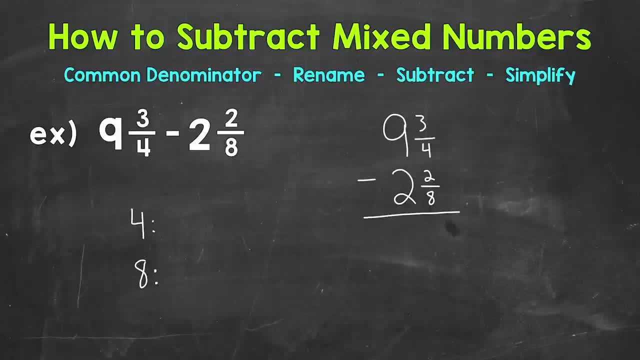 multiple is without writing out the multiples, But I'll write them out as a review. So the multiples of 4, well, let's count up by 4, 4,, 8,, 12,, 16.. Now those multiples go on forever. So my suggestion: write out 4 or 5.. 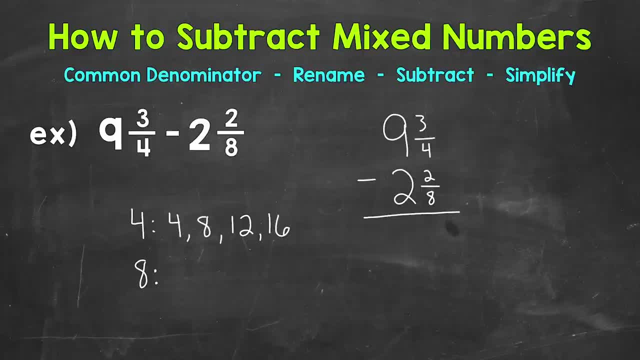 See if you have any in common common. If not, you can always extend your lists. Now let's write out four multiples of 8.. So we have 8,, 16,, 24,, 32.. Once we have that, we can look for the least common multiple which is going to. 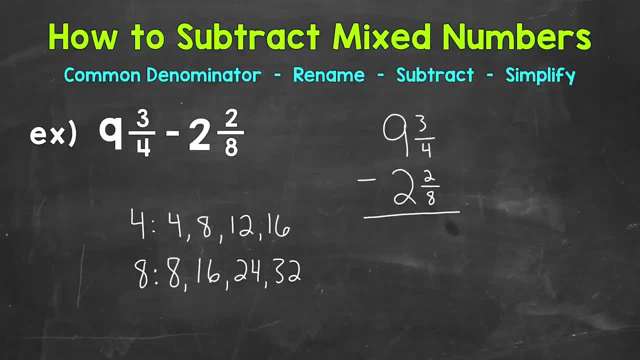 be the smallest number in value that they share, which is going to be 8.. So 8 is going to be our least common denominator. Now that we have the common denominator that we're going to use, we can rename the fractional part of these mixed numbers with that common denominator of 8.. So 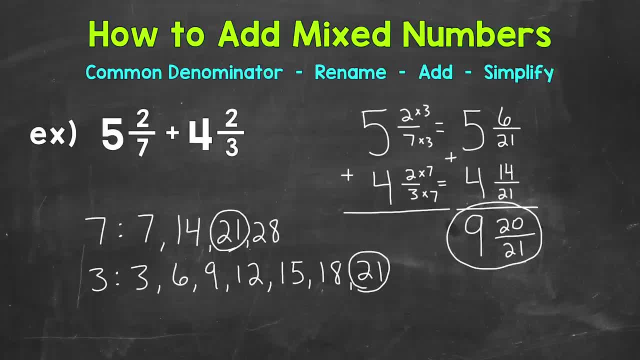 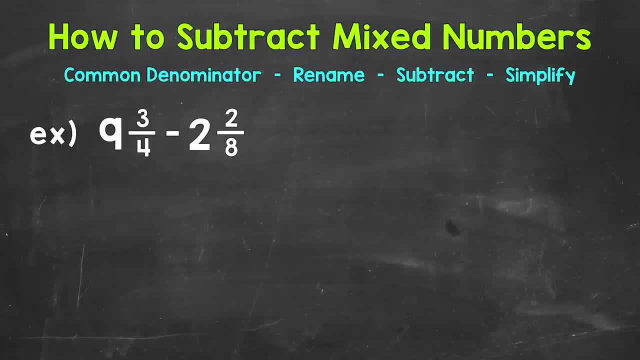 is 9 and 20 21st next let's move on to subtraction so for our subtraction example we have 9 and 21 3 4ths minus 2 and 2 8ths now the first thing that I'm going to do is rewrite this problem vertically so up and down and I'm going to line up my whole numbers and fractions so let's come to the side here and we'll do 9 and 3 4ths minus 2 and 2 8ths so what I'm going to do I'm going to subtract the fractions first so I'm going to subtract the fractions first and then I'm going to and then the whole numbers. Now when we subtract fractions we need a common denominator. So as we have the problem written out now we have a denominator of 4 and a denominator of 8. So we can't subtract quite yet. We need to find a common denominator and rename. We find a common denominator 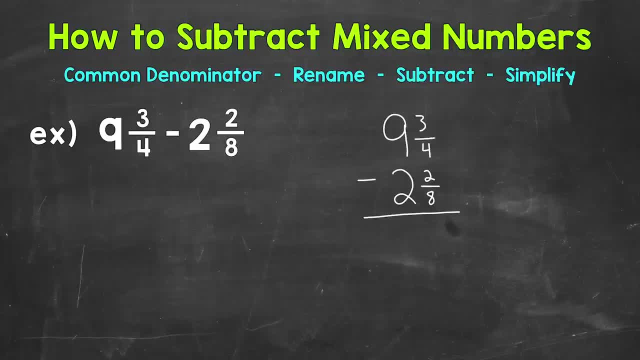 by looking for common multiples and then the least common multiple we can use for our least common denominator. So let's write out our multiples of 4 and 8. Now you may be able to do this figure out what the least common multiple is without writing out the multiples but I'll write them out as a review. So the multiples of 4 well let's count up by 4 4 8 12 16. Now those multiples go on forever so my suggestion write out 4 or 5. 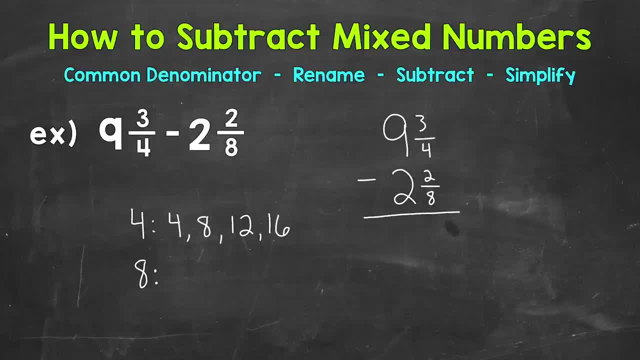 See if you have any in common. If not you can always extend your lists. Now let's write out 4 multiples of 8. So we have 8 16 24 32. Once we have that we can look for the least common multiple 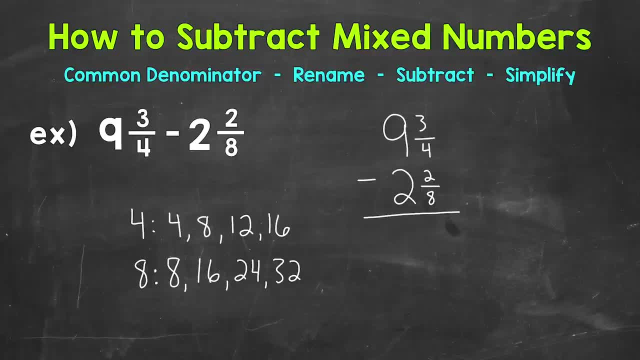 which is going to be the smallest number in value that they share which is going to be 8. So 8 is 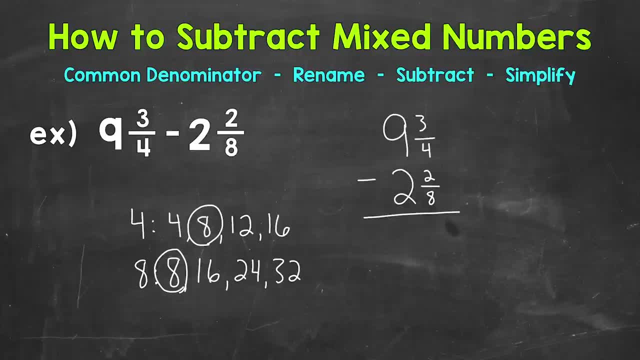 a common denominator. Now that we have the common denominator that we're going to use we can rename the fractional part of these mixed numbers with that common denominator of 8. So let's start with 9 and 3 fourths. So this equals keep our whole number the same and then we need that common denominator of 8. So let's use equivalent fractions here. 4 times 2 equals 8. Now whatever we do to the bottom, we must do to the top in order to keep this equivalent. So 3 times 2 gives us 6. 6 eighths is equivalent to 3 fourths. We're not changing the value of the problem at all. We're just using equivalent fractions to rename that fraction with our common denominator. 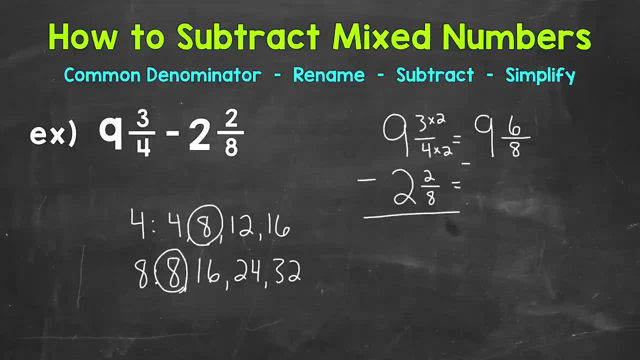 So let's do 2 and 2 eighths now. We'll put our subtraction sign there. Now 2 and 2 eighths, that already has a denominator of 8. So we do not need to do anything with that mixed number, and specifically the fraction. Again, because we already have that denominator of 8. Now that we renamed what we needed to rename, we have a common denominator of 8, and we're able to subtract. So let's subtract the fractions of these mixed numbers. So 6 eighths minus 2 eighths. Subtract the number of fractions. We're able to subtract the fractions of these mixed numbers. So 6 eighths 6 minus 2. That gives us 4. And then we keep our common denominator of 8. Once we have that, we can subtract the whole numbers. So 9 minus 2 gives us 7. So we get 7 and 4 eighths. Always look to see if you can simplify the fractional part of a mixed number. We can. 4 eighths can be simplified. We have a greatest common factor of 4. 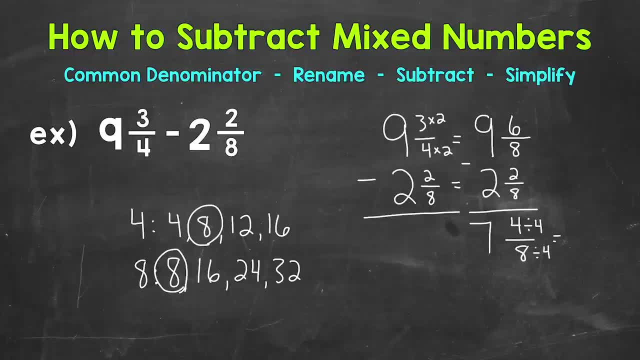 So let's divide both of these by 4. And we get 7. 4 divided by 4 is 1. 8 divided by 4 is 2. So we get a simplified answer of 7 and a half. So we've gone through an addition and a subtraction example. 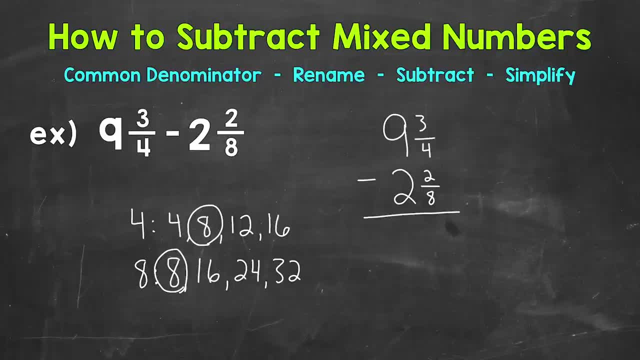 let's start with 9 and 3 fourths, So this equals: keep our whole number the same. and then we need that common denominator of 8. So let's use equivalent fractions here. 4 times 2 equals 8.. 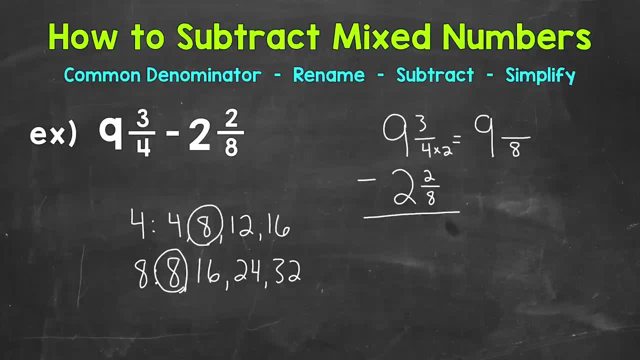 Now, whatever we do to the bottom, we must do to the top in order to keep this equivalent. So 3 times 2 gives us 6.. 6 eighths is equivalent to 3 fourths. We're not changing the value of the. 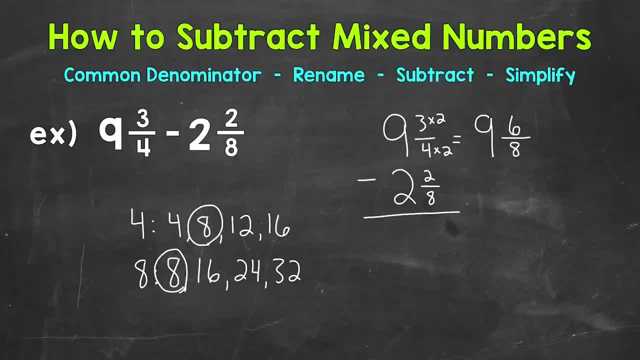 problem at all. We're just using equivalent fractions to rename that fraction with our common denominator. So let's do 2 and 2 eighths. now We'll put our subtraction sign there. Now, 2 and 2 eighths is equivalent to 3 fourths. So let's do 2 and 2 eighths. now We'll put our. 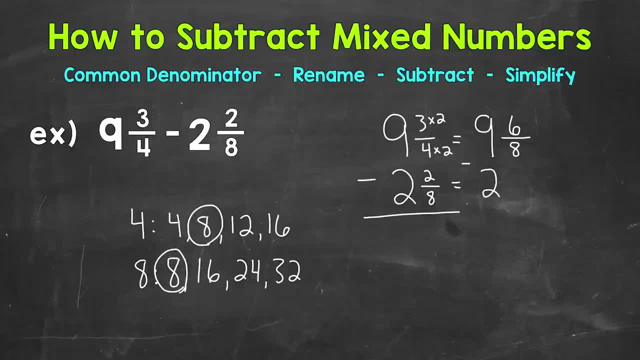 subtraction sign there. Now, 2 and 2 eighths is equivalent to 3 fourths. So let's do 2 and 2 eighths. That already has a denominator of 8.. So we do not need to do anything with that mixed number. 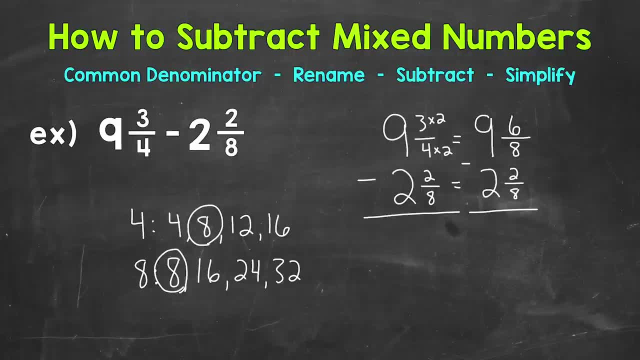 and specifically the fraction Again, because we already have that denominator of 8.. Now that we renamed what we needed to rename, we have a common denominator of 8, and we're able to subtract. So let's subtract the fractions of these mixed numbers, So 6 eighths minus 2 eighths. 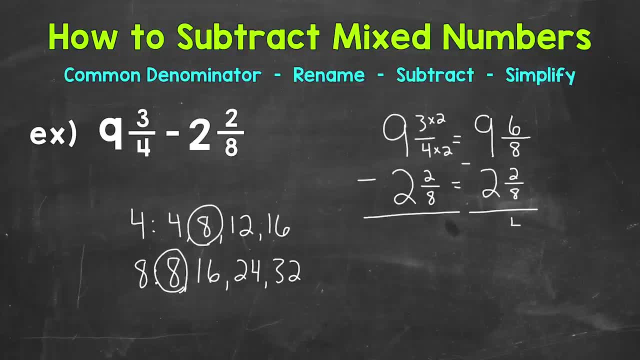 Subtract the numerators 6 minus 2.. That gives us 4.. And then we keep our common denominator of 8. Once we have that, we can subtract the whole numbers. So 9 minus 2 gives us 7.. So we get 7 and 4 eighths. 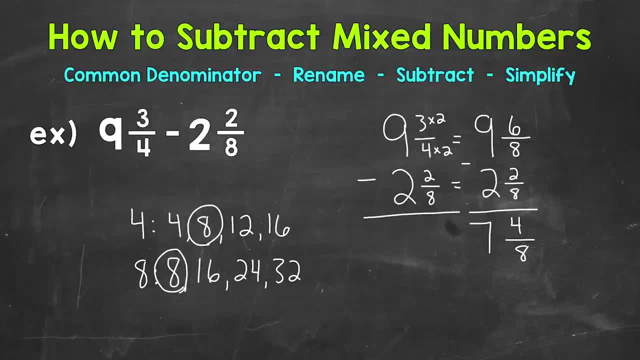 Always look to see if you can simplify the fractional part of a mixed number. We can. 4 eighths can be simplified. We have a greatest common factor of 4.. So let's divide both of these by 4. And we get 7.. 4 divided by 4 is 1.. 8 divided by 4 is 2.. 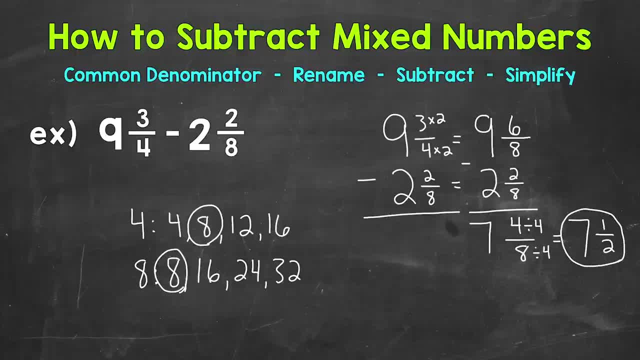 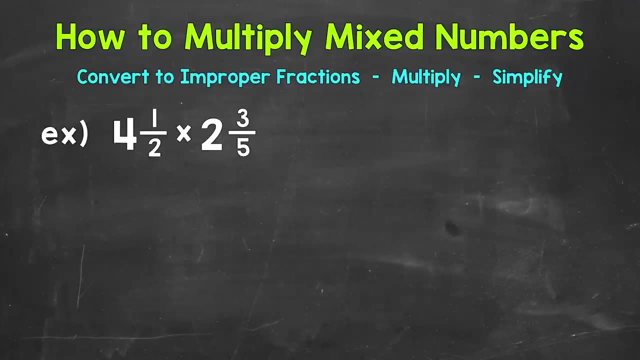 So we get a simplified answer of 7 and a half. So we've gone through an addition and a subtraction example. Now we'll move on to multiplication. For our multiplication example we have 4 and a half times 2 and 3 fifths. 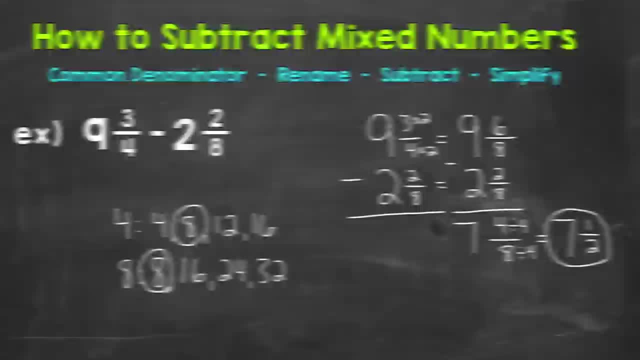 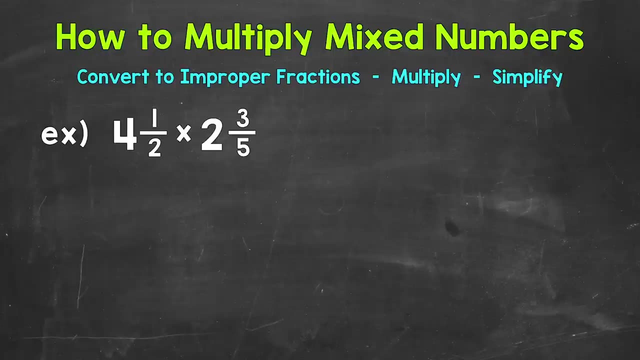 Now we'll move on to multiplication. For our multiplication example, we have 4 and a half times 2 and 3 fifths. Now the first thing that we want to do is to convert our mixed numbers to improper fractions. That way we have a numerator and a denominator and we can multiply straight across. So in order to do this, we start at the bottom. So let's start at the bottom here and we work our way to the top. We multiply, then add. So we do 2 times 4, our denominator times the whole number. So 2 times 4 is 8 plus our numerator of 1. That gives us 9. So again, 2 times 4 is 8 plus 1 gives us 9. That's the 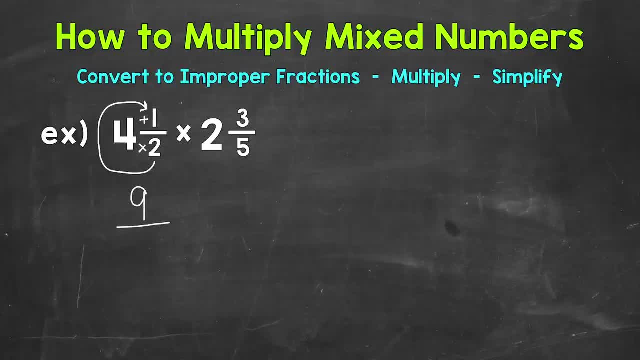 numerator of our improper fraction. We keep our denominator of 2 the same. Now that improper fraction is equivalent to our mixed number. They're just in different forms. We're not changing the value of the problem at all when we convert to an improper fraction. 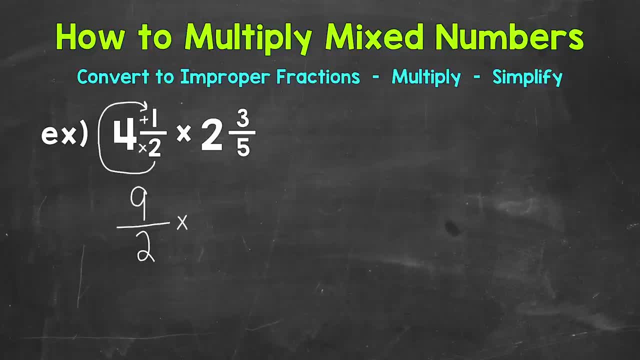 Let's bring our multiplication sign down and then convert our other mixed number. So we multiply, then add. 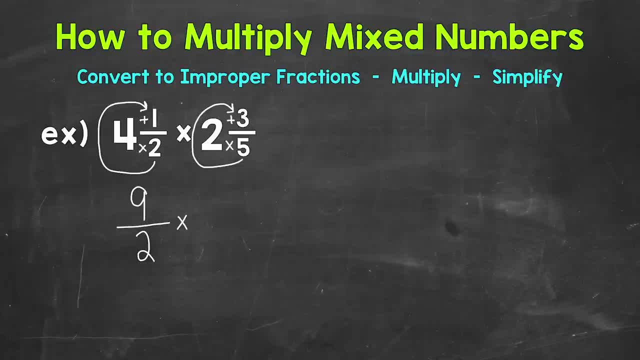 So 5 times 2 is 10 plus 3 gives us 13. That's our numerator. And then keep our denominator of 5 the same. 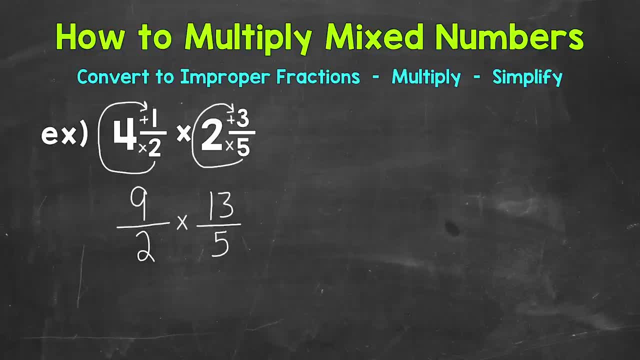 Once we have our mixed numbers converted to improper fractions, we can multiply straight across. So numerator times numerator and denominator. Once we have our mixed numbers converted to improper fractions, we can multiply straight across. So numerator times numerator and denominator. Once we have our mixed numbers converted to improper fractions, we can multiply straight across. So numerator times denominator and denominator. 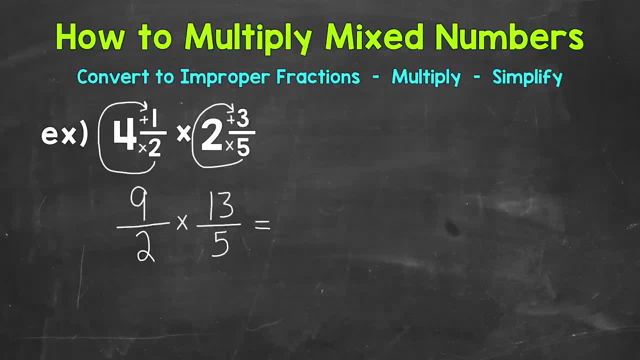 Let's start with the numerators. So 9 times 13, that gives us 117. And then 2 times 5 gives us 10. So that's our answer as an improper fraction, 117 tenths. Now let's convert that to a mixed number. We do that by dividing our numerator 117 by 10. Now we can either do this using mental math, Or writing out the division problem to the side. I'll do both here. 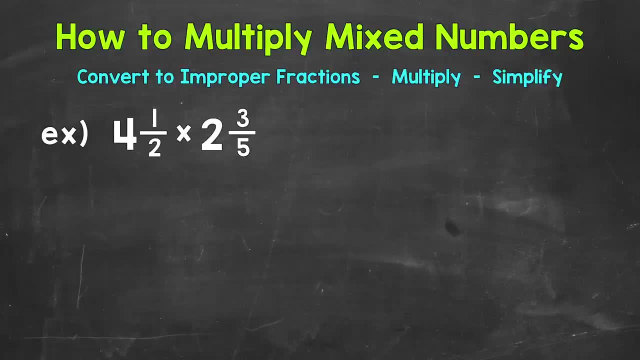 Now the first thing that we want to do is to convert our mixed numbers to improper fractions. That way, we have a numerator and a denominator and we can multiply straight across. So in order to do this, we start at the bottom. So let's start at the bottom here And we work our way. 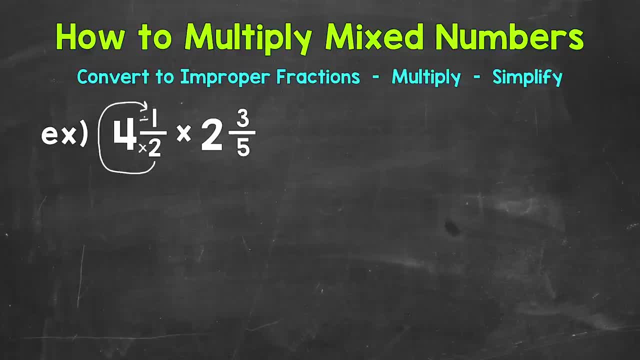 to the top. We multiply, then add. So we do 2 times 4, our denominator times the whole number, So 2 times 4.. We multiply, then add. So 2 times 4 is 8, plus our numerator of 1. That gives us 9.. So again, 2 times 4 is 8, plus 1 gives us 9.. 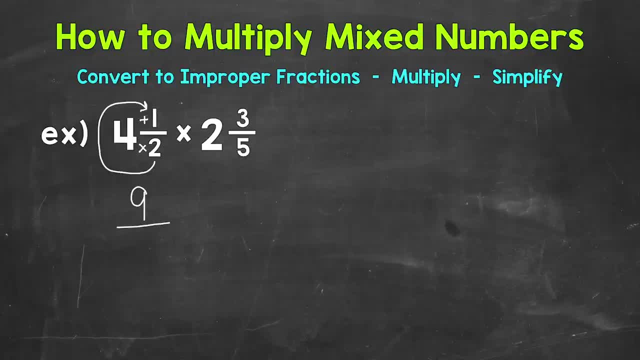 That's the numerator of our improper fraction. We keep our denominator of 2 the same, Now that improper fraction is equivalent to our mixed number. They're just in different forms. We're not changing the value of the problem at all when we convert to an improper fraction. 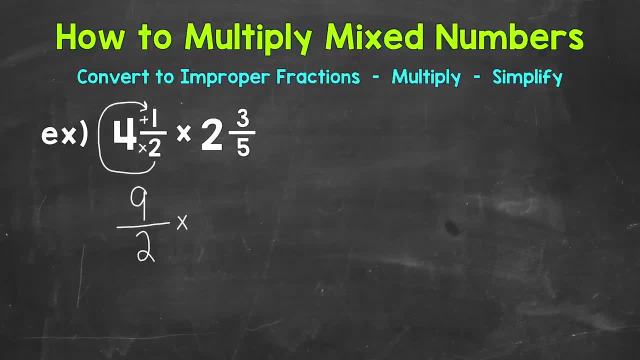 Let's bring our multiplication sign down and then convert our other mixed number So we multiply, then add. So 5 times 2 is 10, plus 3 gives us 13.. That's our numerator, And then keep our denominator of 5 the same. 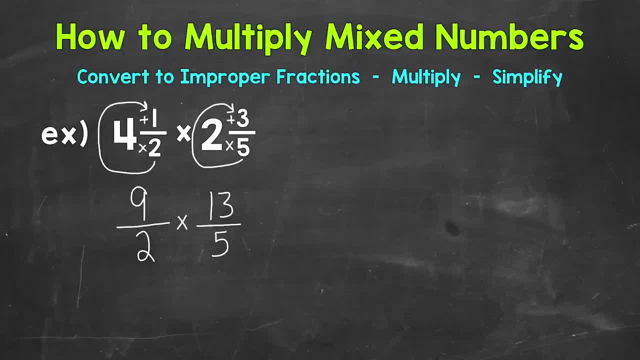 Once we have our mixed numbers converted to improper fractions, we can multiply straight across. So numerator times numerator and denominator. So numerator times numerator and denominator. denominator times denominator. Let's start with the numerators. So 9 times 13.. That gives us 117.. 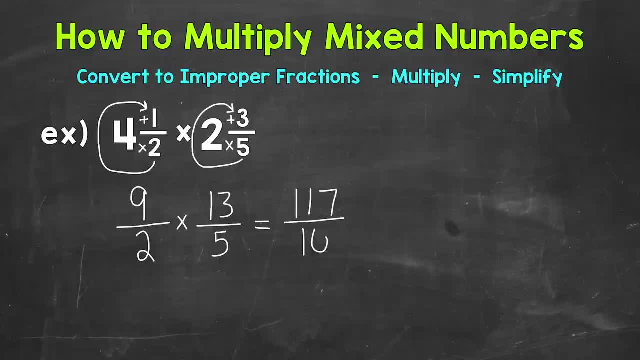 And then 2 times 5 gives us 10.. So that's our answer as an improper fraction: 117 tenths. Now let's convert that to a mixed number. We do that by dividing our numerator- 117, by 10.. Now, we can either do this using mental math, or we can do this by dividing our numerator 117, by 10.. Now we can either do this using mental math, or we can do this by dividing our numerator 117, by 10.. 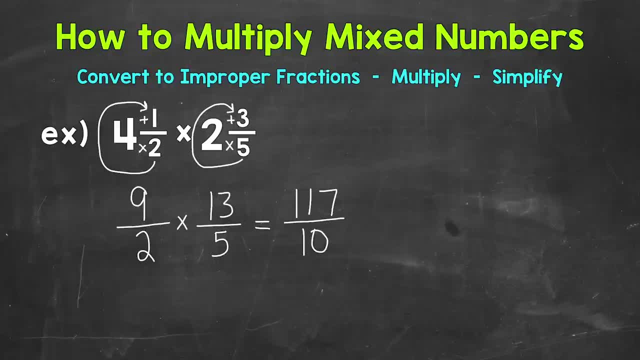 or writing up the division problem to the side. I'll do both. So 117 divided by 10.. How many whole groups of 10 can we pull out of 117?? Well, 11!. That parts u 2 equals 110.. 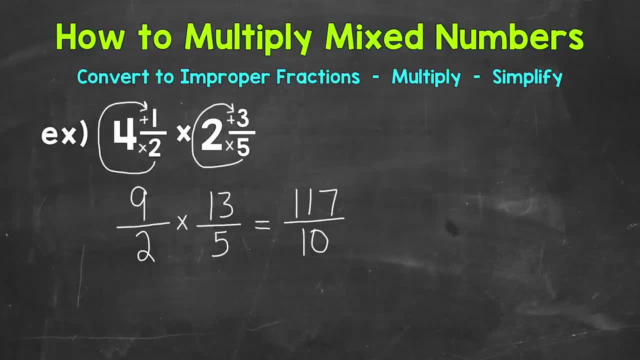 So 117 divided by 10. How many whole groups of 10 can we pull out of 117? Well, 11. That gets us to 110. We don't hit 117 exactly. So we have something left over, a remainder. So the difference between 110 and 117 is 7. That's what's left over. 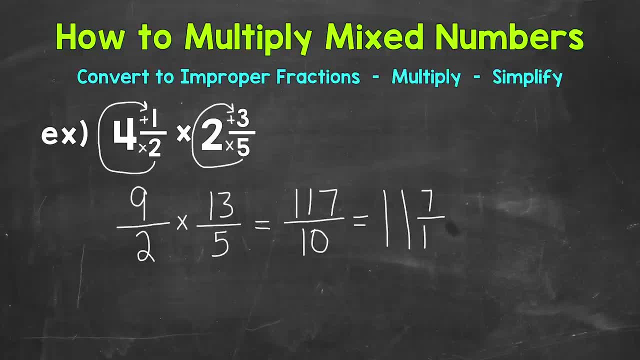 That's our numerator. And then keep our denominator of 10 the same. 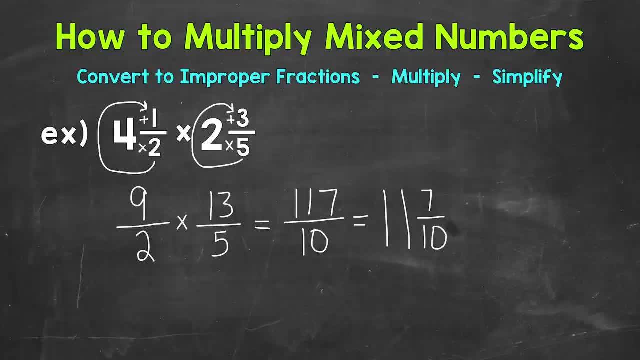 Now, if you're unable to do that using mental math, you can always come to the side and write out the division problem. 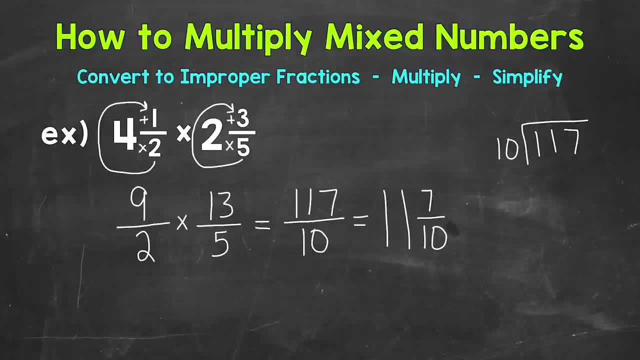 So for example, we'll start with how many whole groups of 10 out of 11? 1. 1 times 10 is 10. Subtract. We get 1. 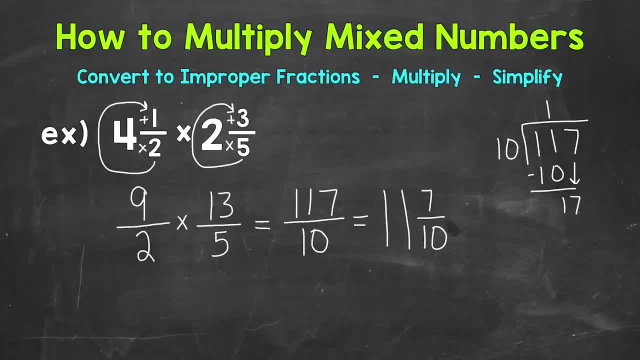 Bring down the 7. So how many whole groups of 10 out of 17? 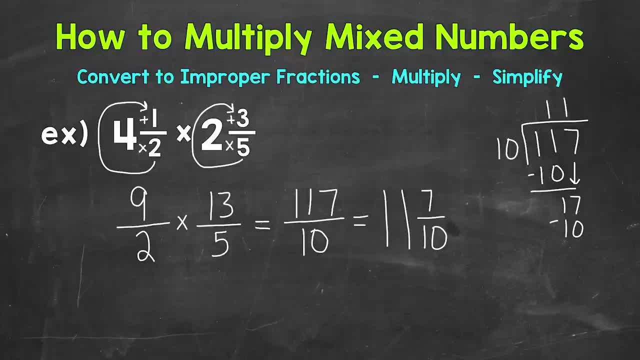 1. 1 times 10 is 10. Subtract. And we get a remainder of 7. So we get the same thing either way. 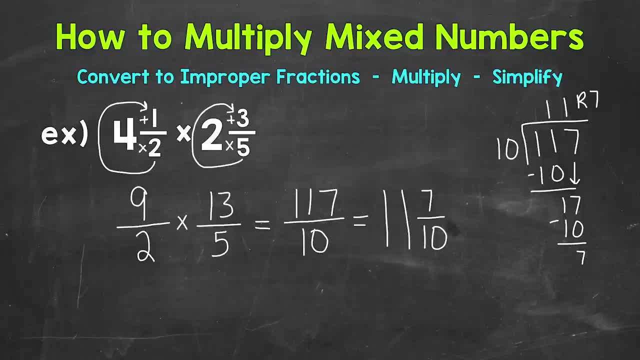 Sometimes problems are a little more friendly and we can do them using mental math. Sometimes we may need to write out the division problem. Either way works. 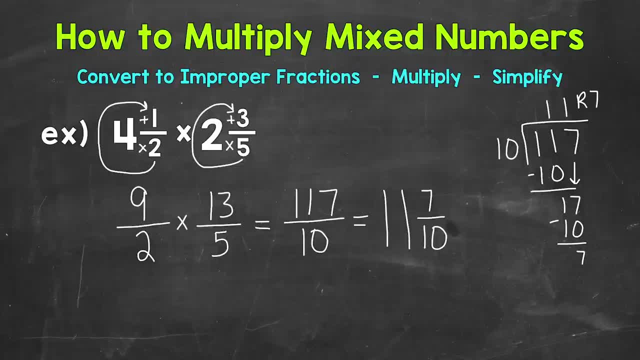 So just to recap how we converted from an improper fraction to that mixed number, we did 117, the numerator, divided by 10, the denominator. So how many whole groups? Whole groups of 10 out of 117. 11. Then we have a remainder of 7, which is our numerator, and we keep our denominator of 10 the same. Always check to see if you can simplify the fractional part of a mixed number. 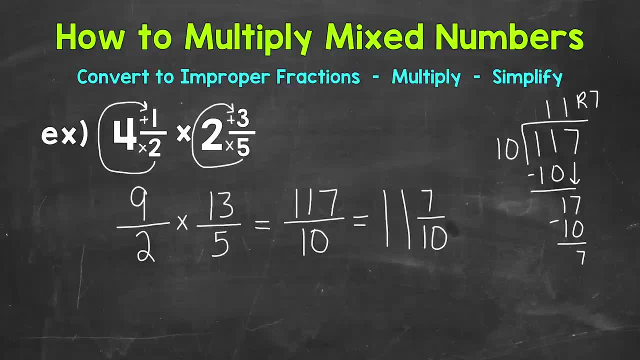 Well, 7 tenths is in simplest form. The only common factor between 7 and 10 is 1. So this is in simplest form. 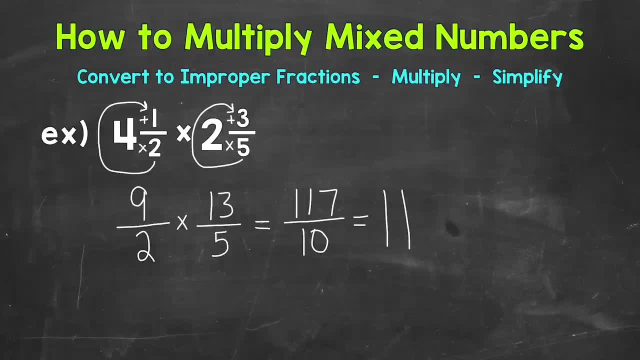 We don't hit 117 exactly, so we have something left over, A remainder. So the difference between 110 and 117 is 7.. That's what's left over, left over. That's our numerator. And then keep our denominator of 10 the same. Now, if you're. 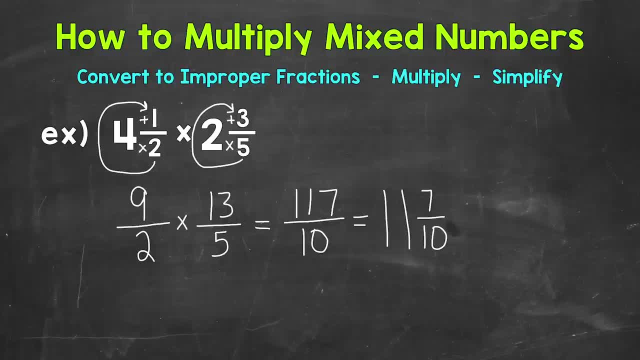 unable to do that using mental math, you can always come to the side and write out the division problem. So, for example, we'll start with how many whole groups of 10 out of 11? One One times 10 is 10.. Subtract We get 1.. Bring down the 7.. So how many whole groups of 10 out of 17? One One times 10. 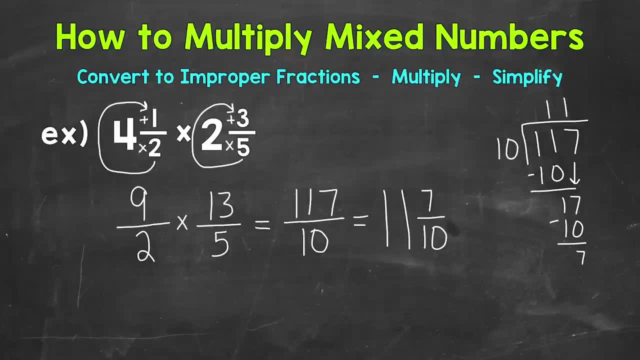 is 10.. Subtract And we get a remainder of 7. So we get the same thing either way. Sometimes problems are a little more friendly and we can do them using mental math. Sometimes we may need to write out the division problem. Either way works. So just to recap how we converted: 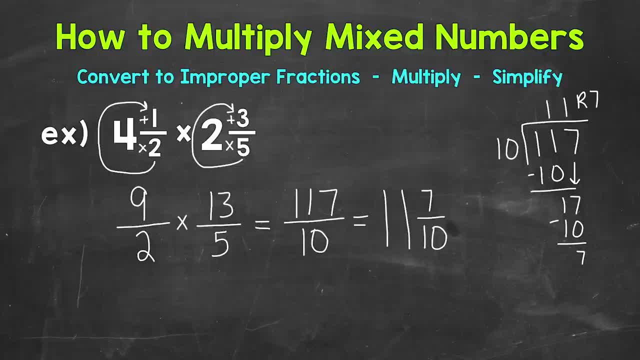 from an improper fraction to that mixed number. we did 117, the numerator divided by 10, the denominator. So how many whole groups of 10 out of 117? 11.. Then we have a remainder of 7,, which is 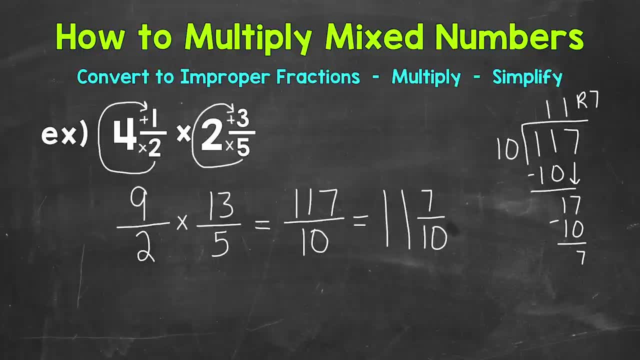 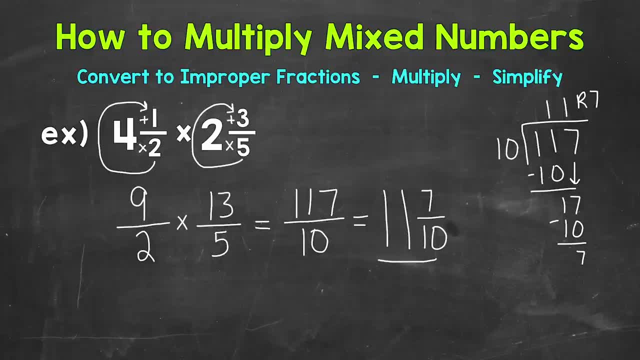 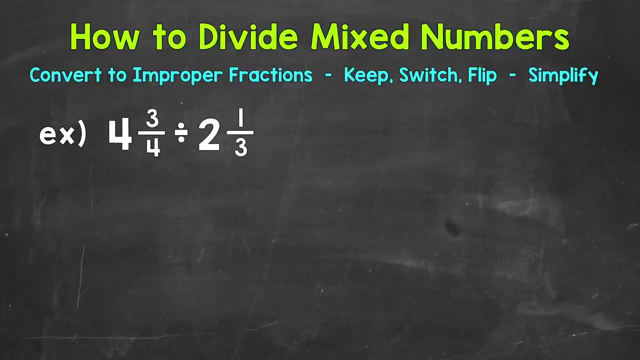 7 and 10 is 1.. So this is in simplest form And we are done: 11 and 7 tenths. Lastly, let's move on to division. So for our division example, we have 4 and 3 fourths. 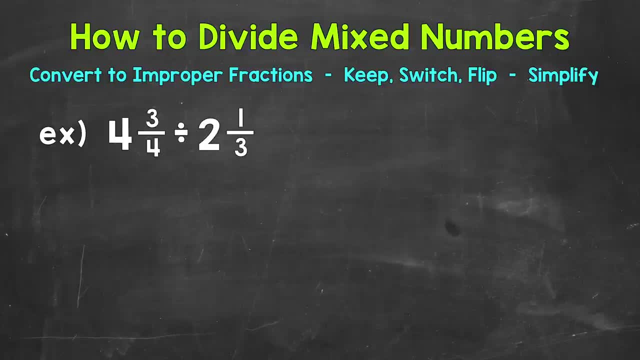 divided by 2 and 1. third. Now, the first thing that we want to do is to convert these mixed numbers to improper fractions. That way we just have a numerator and a denominator. Let's start with 4 and 3, fourths, And we start at the bottom and work our way to the top. So we 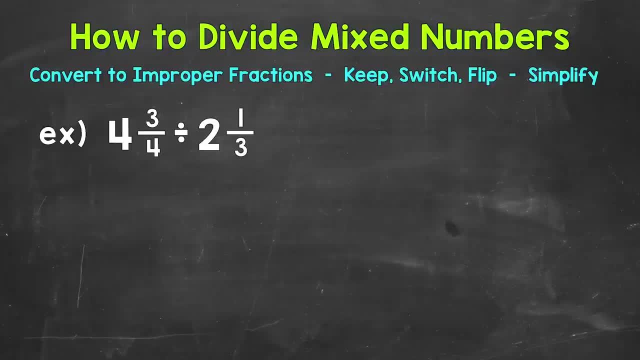 Lastly, let's move on to division. So for our division example, we have 4 and 3 fourths divided by 2 and 1 third. Now the first thing that we want to do is to convert these mixed numbers to improper fractions. That way we just have a numerator and a denominator. 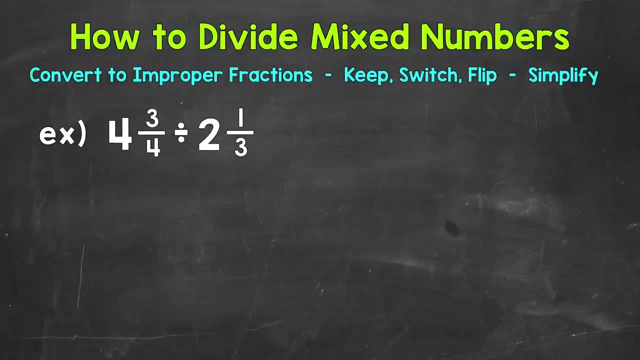 Let's start with 4 and 3 fourths. And we start at the bottom and work our way to the top. So we multiply, then add. So we do 4 times 4, so the denominator times the whole number. 4 times 4 is 16. Then we add the numerator. 16 plus 3 is 19. So 19 is the numerator of our improper fraction. We keep our denominator of 4 the same. 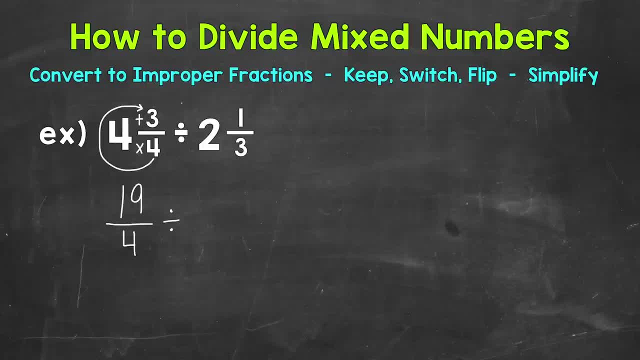 Then we can bring our division sign down and convert. Our second mixed number. So again, we multiply, then add. So 3 times 2 is 6. Plus 1 is 7. That's our numerator. And then keep the denominator of 3 the same. So 7 thirds. 19 fourths is equivalent to 4 and 3 fourths. 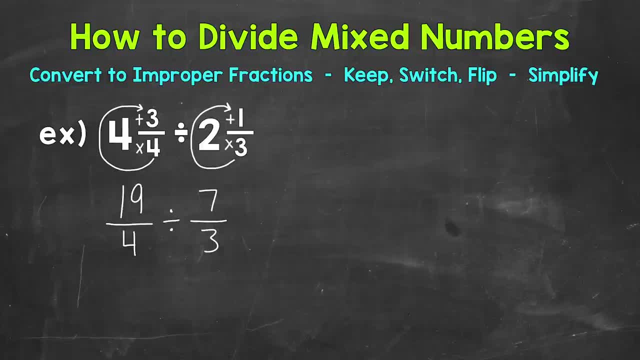 And then 7 thirds is equivalent to 2 and 1 third. 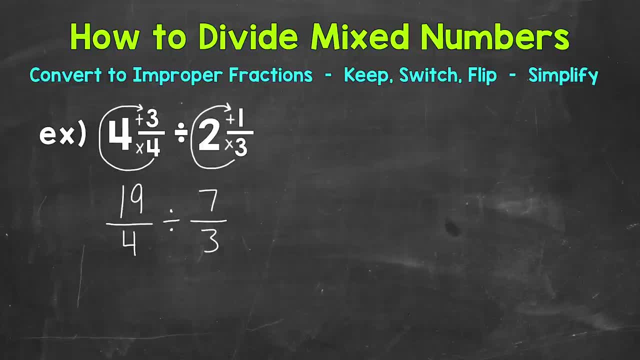 So we're not changing the value of the problem at all. When we convert to improper fractions. 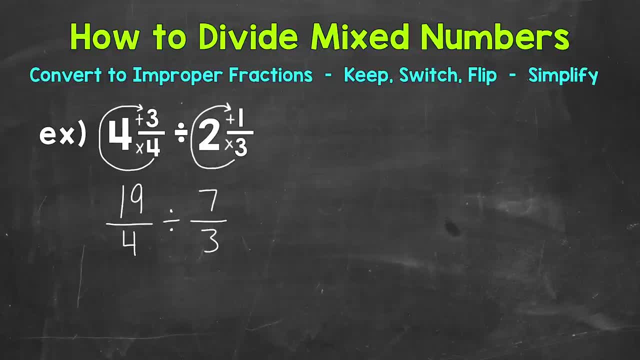 Mixed numbers and improper fractions are equivalent. They're just in different forms. 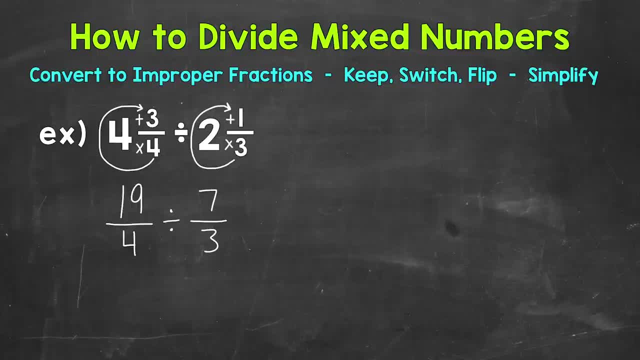 Now again, we're converting to improper fractions. So we just have a numerator and a denominator. And then we can go through our steps for dividing these fractions. Which we're going to use keep, switch, flip. 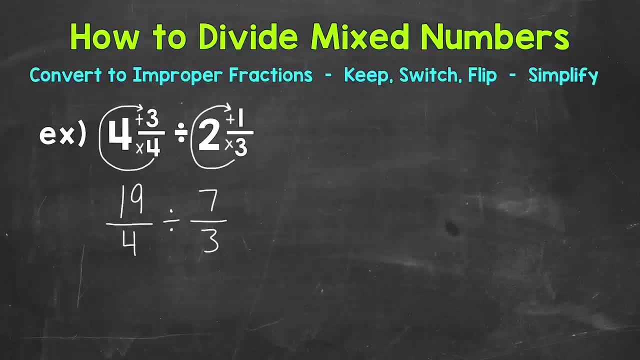 Also known as keep, change, flip. So no matter how you think of it, they mean the same thing. 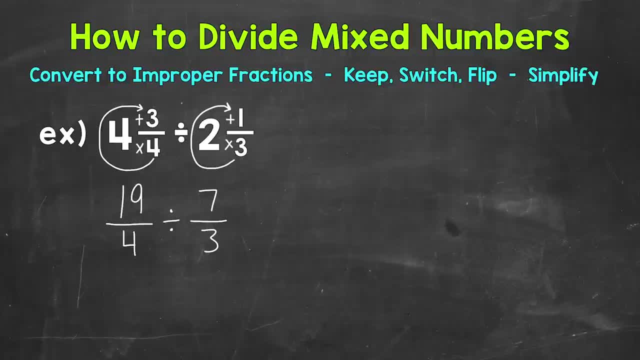 I know there's different words out there. For these steps, but in the end, they all mean the same thing. 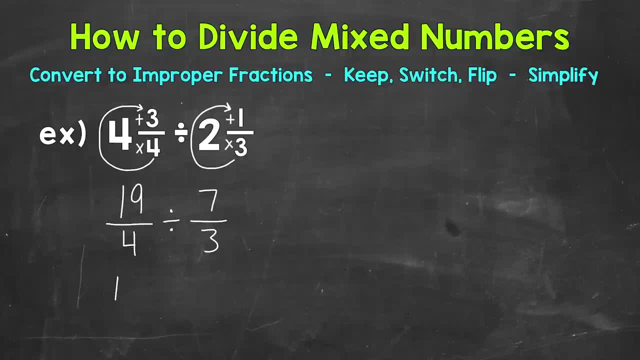 So let's keep our first fraction here. Our first improper fraction. So 19 fourths. Then we switch or change our division to multiplication. And then we flip our second fraction. 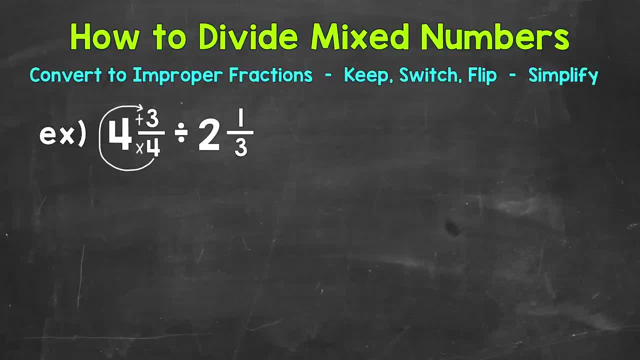 multiply, then add. So we do 4 times 4.. So the denominator times the whole number 4 times 4 is 16.. Then we add the numerator 16 plus 3 is 19.. So 19 is the numerator of our improper fraction. 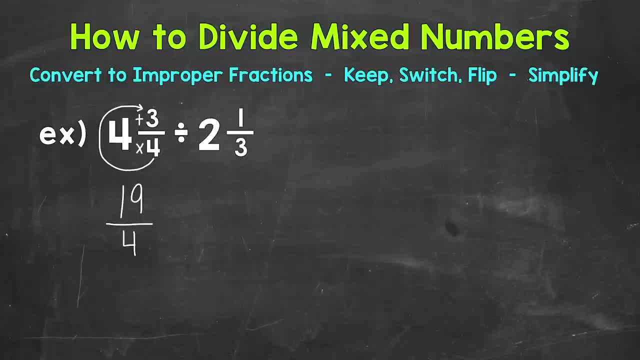 We keep our denominator and our denominator. We keep our numerator and our denominator. We keep denominator of 4, the same. then we can bring our division, sign down and convert our second mixed number. so again we multiply, then add. so 3 times 2 is 6 plus. 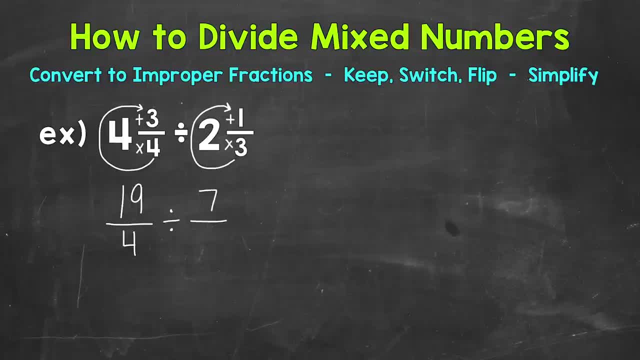 1 is 7. that's our numerator, and then keep the denominator of 3 the same. so 7 thirds, 19 fourths, is equivalent to 4 and 3 fourths, and then 7 thirds is equivalent to 2 and 1 third. so we're not changing the value of the problem at all. 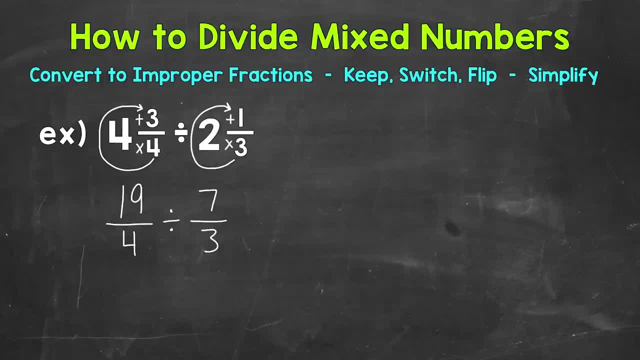 when we convert to improper fractions. mixed numbers and improper fractions are equivalent, they're just in different forms. now again, we're converting to improper fractions, so we just have a numerator and a denominator, and then we can go through our steps. for the next step, so we're going to use keep switch flip, also known as keep change flip. so no, 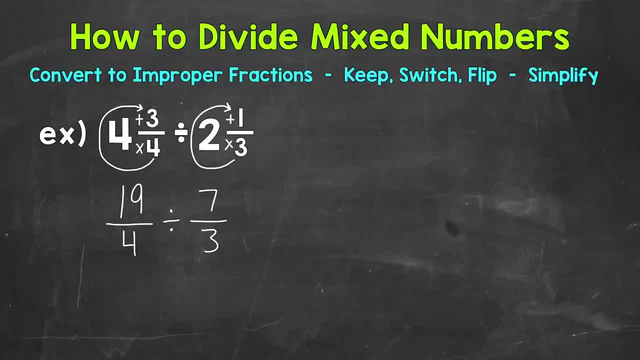 matter how you think of it, they mean the same thing. I know there's different words out there for these steps, but in the end they all mean the same thing. so let's keep our first fraction here, our first improper fraction, so 19 fourths. then we switch or change our division to multiplication and then we're going to. 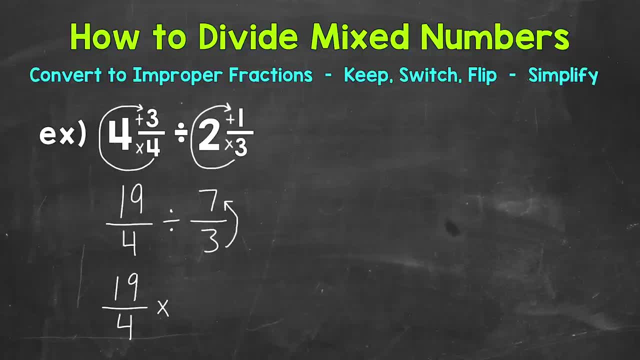 flip our second fraction, our second improper fraction here. so the denominator becomes the numerator and the numerator becomes the denominator. this is called the reciprocal. so we have 3- 7ths. once we get to this point we can multiply straight across. so numerator times numerator and then denominator. 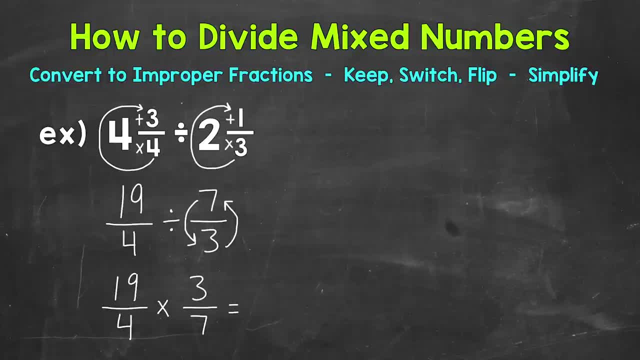 times denominator. let's do the numerators. first times 3, that gives us 57, and then we have 4 times 7, which is 28.. Now that's our answer. as an improper fraction, We're going to convert it to a mixed number. so 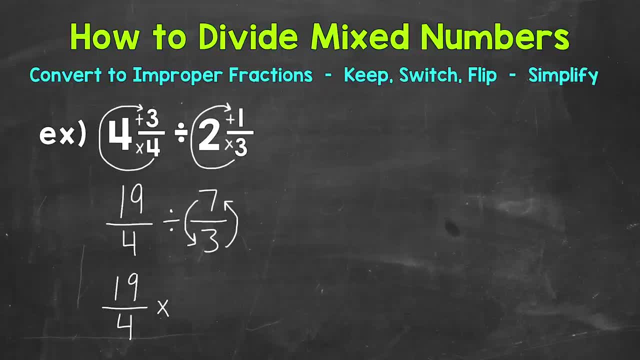 Our second improper fraction here. So the denominator becomes the numerator. And the numerator becomes the denominator. And the numerator becomes the denominator. This is called the reciprocal. 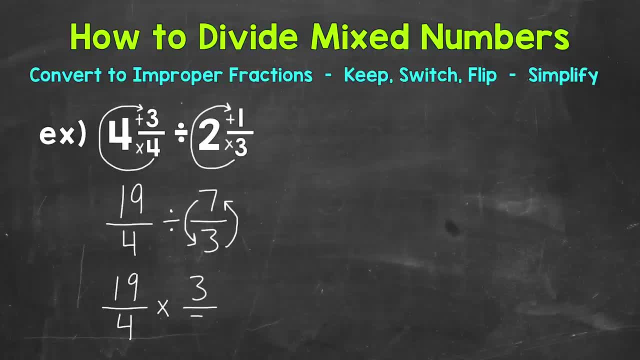 So we have 3 sevenths. Once we get to this point, we can multiply straight across. So numerator times numerator. And then denominator times denominator. 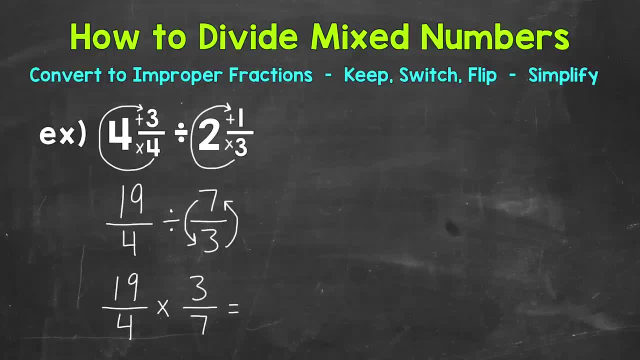 Let's do the numerators first. So 19 times 3. That gives us 57. 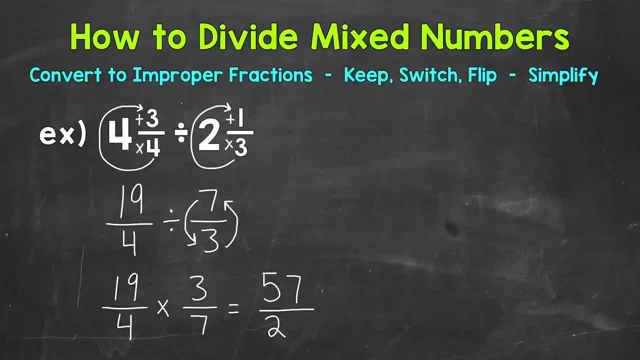 And then we have 4 times 7. Which is 28. 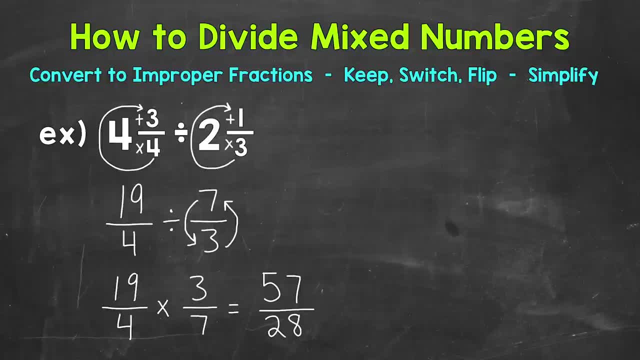 Now that's our answer as an improper fraction. We're going to convert it to a mixed number. So we need to do our numerator, 57. Divided by our denominator, 28. 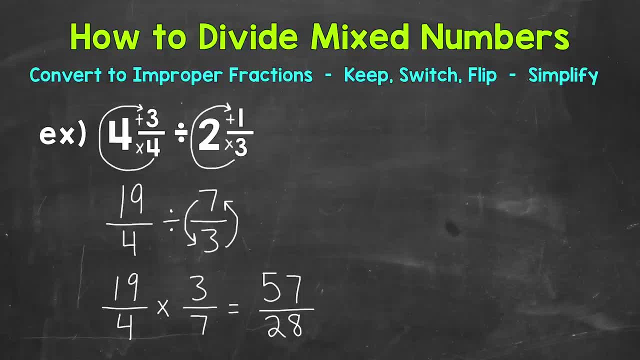 Now we can do this using mental math. Or we can write everything out. 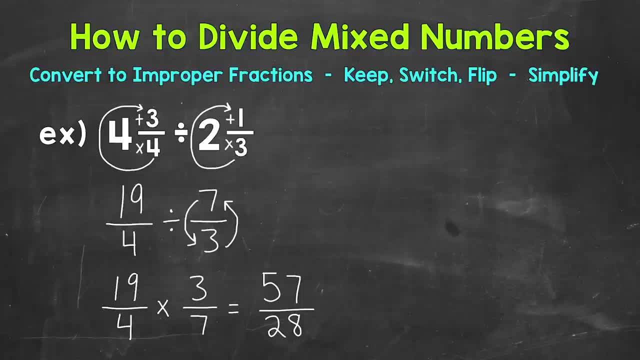 Some problems are going to be a little simpler. And we're going to be able to use mental math. And in some situations, we'll have to write out the problem. 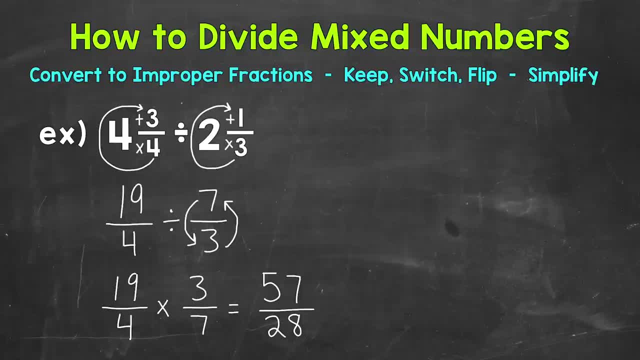 I'll go through both here so you can see what that looks like. Let's use mental math here first. So how many whole groups of 28 are there? How many whole groups of 28 out of 57? Well, if you're able to think about that. 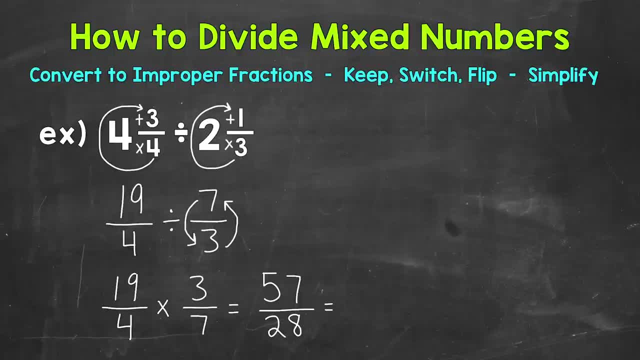 It's going to be 2 whole groups of 28. Because that gets us to 56. So 2 whole groups of 28. Now we do not hit 57 exactly. We have something left over. A remainder. So the difference between 57 and 56 is 1. So we have a remainder of 1. And we keep our denominator of 28. 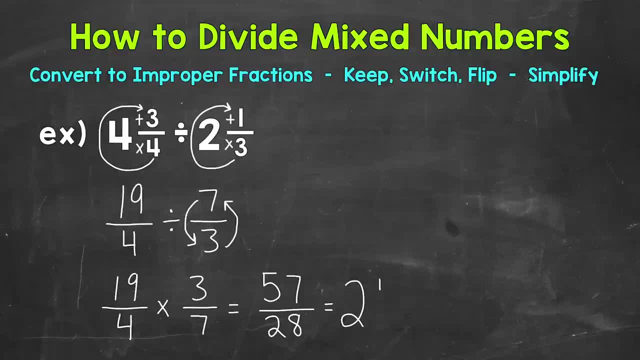 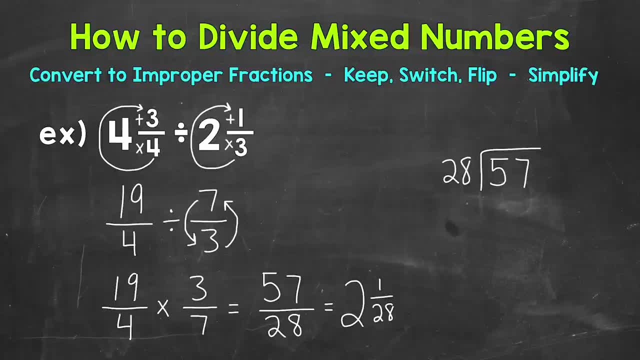 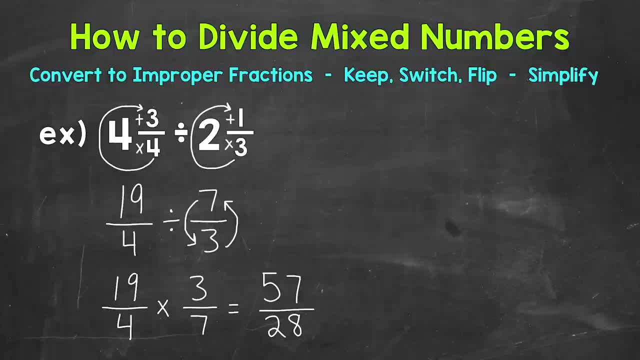 we need to do our numerator 57 divided by our denominator 28.. Now we can do this using mental math or we can write everything out. Some problems are going to be a little simpler and we're going to be able to use mental math and in 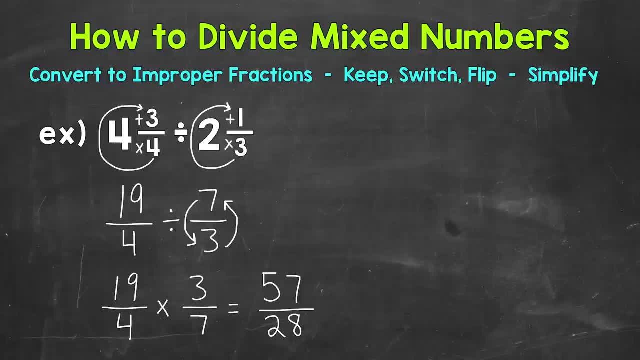 some situations we'll have to write out the problem. I'll go through both here so you can see what that looks like. Let's use mental math here first. So how many whole groups of 28 out of 57?? Well, if you're able to think about that, it's. 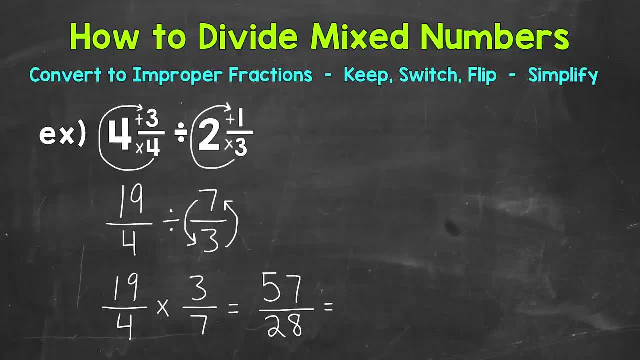 going to be two whole groups of 28, because that gets us to 56. So two whole groups of 28.. Now we do not hit 57 exactly. we have something left over, a remainder. So the difference between 57 and 56 is 1. 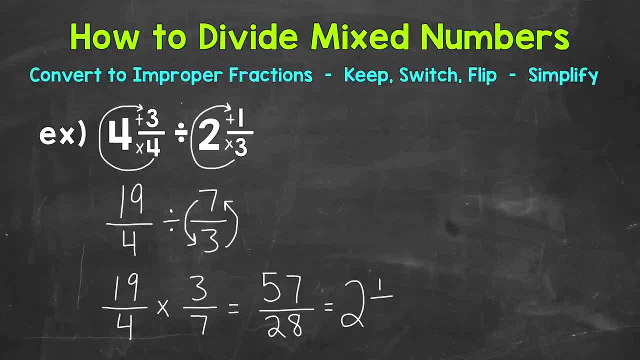 so we have a remainder of 1 and we keep our denominator of 28 the same. Let me write that out as well. So we have 57 divided by 28.. So we need to think how many whole groups of 28 out of 57. Well, we said that's 2.. That gets us to 56. so 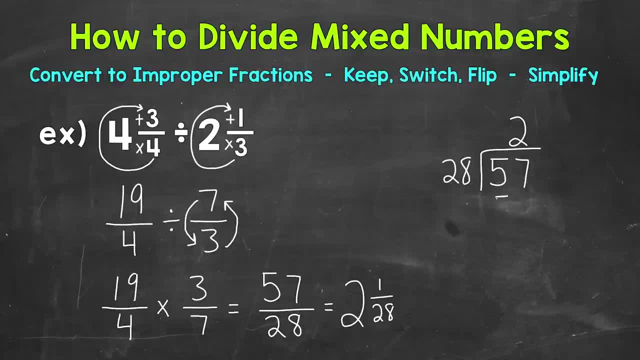 2. 2 times 28 is 56. So we get a remainder of 1.. This 2 is going to be the whole number, part of our mixed number. 2 whole 28's out of 57, and then this 1, the remainder is going to be the numerator, and then we keep our. 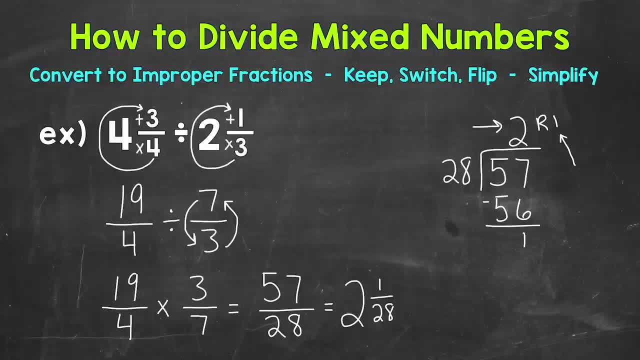 denominator of 28 the same. Once we get to our mixed number, we can check to see if we can simplify the fractional part. 1- 28th is in simplest form: The only common factor between 1 and 28 is 1, so we are done 2 and 1- 28th. So there you have it. There's a review of 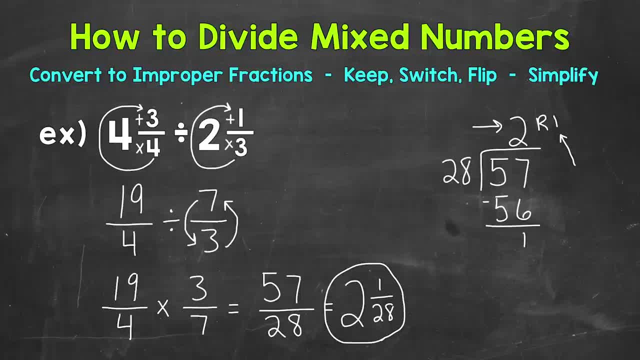 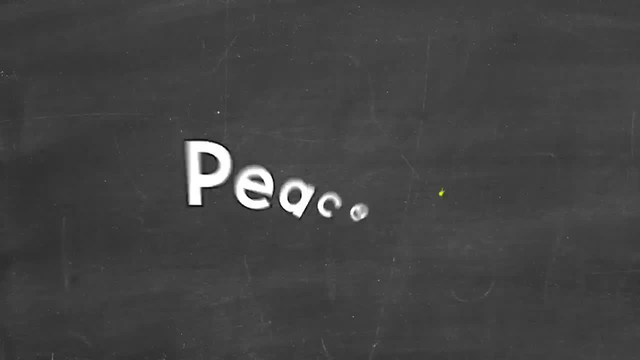 how to add, subtract, multiply and divide mixed numbers. I hope that helped. Thanks so much for watching. Until next time, peace.